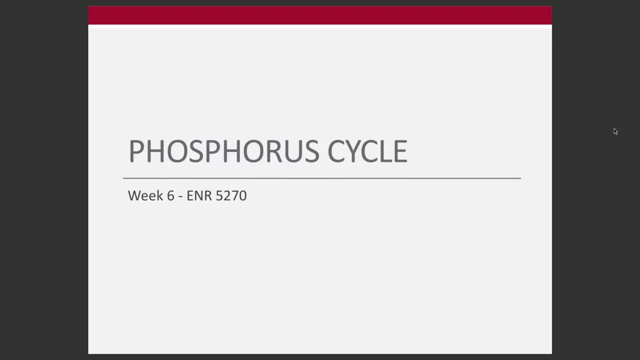 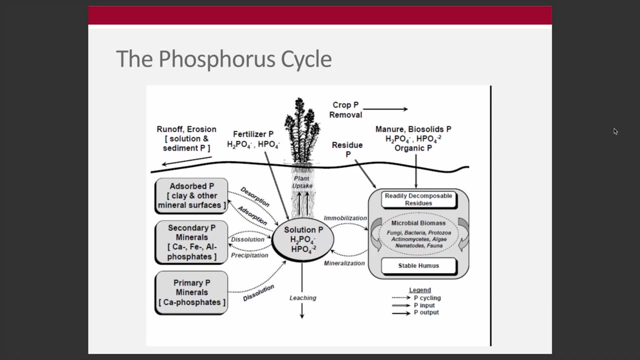 Next up is the phosphorus cycle. There's a fair amount of slides here, so let's go ahead and get started. Okay, so here is a phosphorus cycle and it looks hopefully somewhat familiar regarding, say, nitrogen or some of the other cycles that we'll deal with, but there's several. 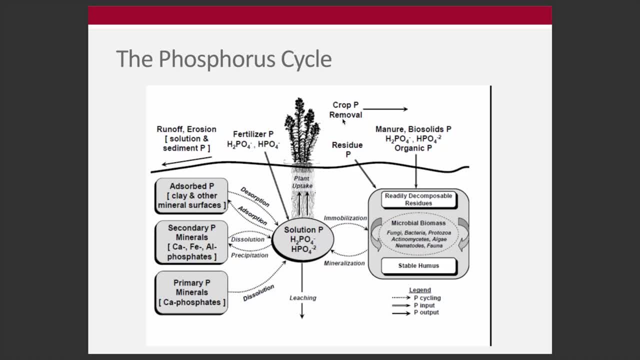 pieces to this. There's additions, things like fertilizer, for example, plant residue, manure or biosolids that are going in. There's this organic fraction, organic form of phosphorus, which includes residues, the microbial biomass, all of the organisms present in the soil, this 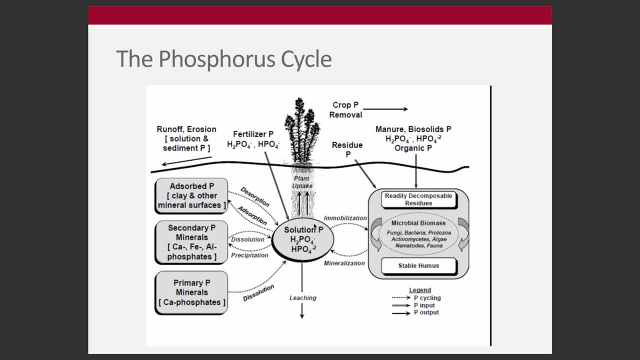 stable humus. And then, of course, on the left, here is the inorganic fraction, so things like clay minerals and secondary minerals, et cetera, et cetera. So we're going to get into each one of these pieces. Losses include things. 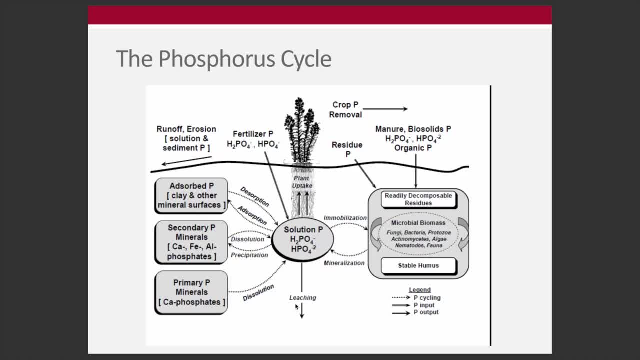 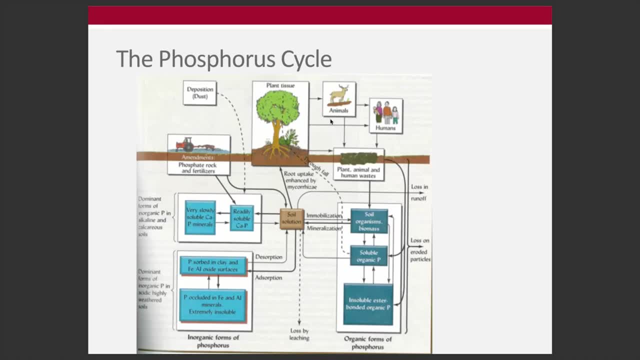 like runoff and erosion, a little bit of leaching- that occurs with phosphorus- and then, of course, crop removal. Here's another picture. The first picture was from the Haviland textbook. This is from the Brady and Wiles. This is the Haviland textbook. This is from the Brady and Wiles. 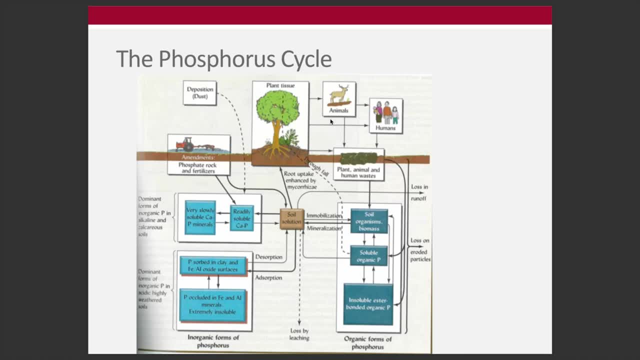 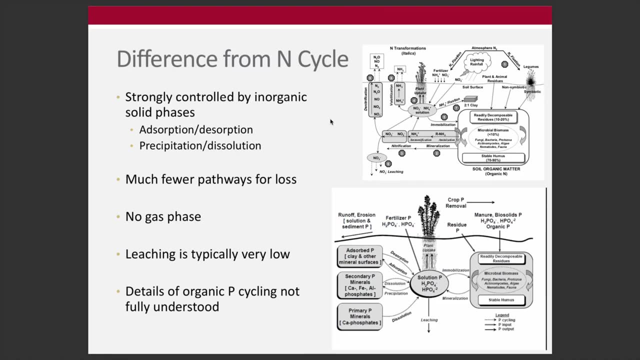 This is the Haviland textbook. This is the Haviland textbook. It's the same pieces, but maybe just might just help to kind of look at it in a little bit different function or format. We can compare and contrast the phosphorus cycle with the nitrogen cycle. 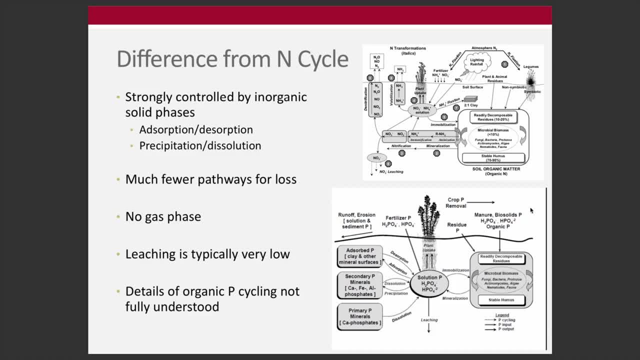 and we'll see that, the nitrogen cycle being up here that we've already discussed, and the phosphorus cycle we just introduced, and there's some differences. So one of the main differences is that this whole inorganic fraction or inorganic phase that's strongly controlled by adsorption and desorption, reactions or precipitation, and 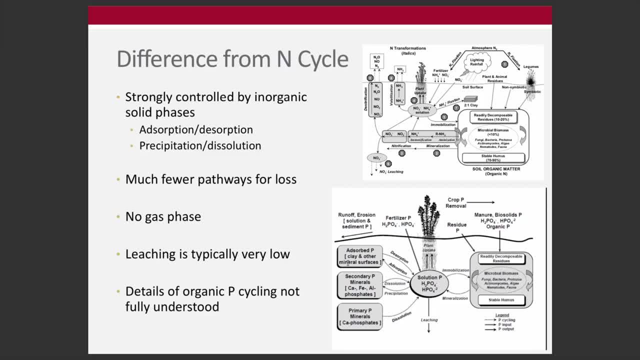 dilution reactions. So that's represented by these boxes here. And notice that in phosphorus that's not present at all in the nitrogen cycle. We'll see that, for phosphorus has much fewer pathways for loss. So for nitrogen we have leaching, denitrification, volatilization And 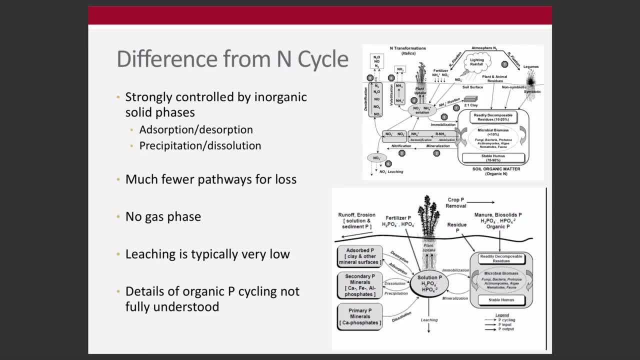 here there's also erosion, which didn't even make its way to the chart. Here we just really have erosion and then a small amount of leaching. that's possible. There's no gaseous phase in phosphorus, unlike nitrogen. Leaching rates are typically very low for phosphorus compared to nitrogen. 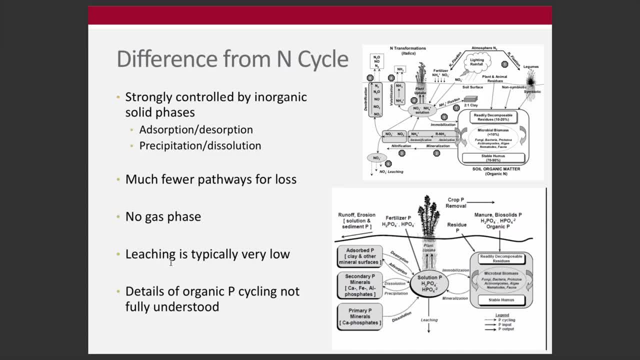 Nitrogen we can get a large amount of total N that's left. It's not uncommon to see 20,, 30, maybe 40 kilograms of nitrogen. There's a lot of nitrogen that are lost in nitrate in a fertilized system. But for phosphorus? 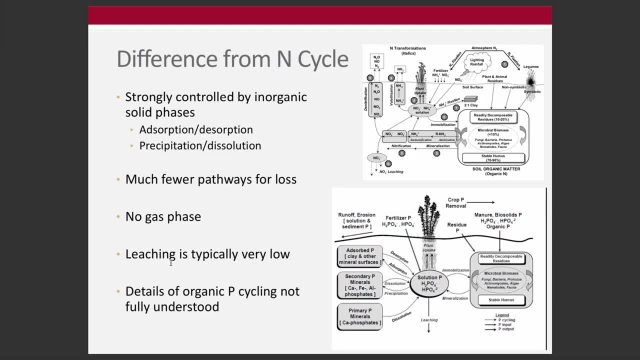 those would be at least maybe one or two kgs or something like that. So like an order of magnitude, less than we're talking, and maybe even less than that than we're talking with nitrogen- Another piece that I won't really get into, but details of organic phosphorus. cycling is not 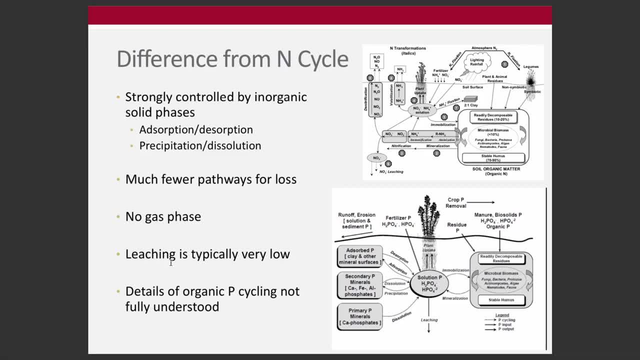 particularly understood, And part of that is because it's very difficult to study phosphorus and organic phosphorus cycling. We don't have methodologically very good tools to do that. For nitrogen, we've got stable isotope forms of nitrogen which are very have become really commonplace. 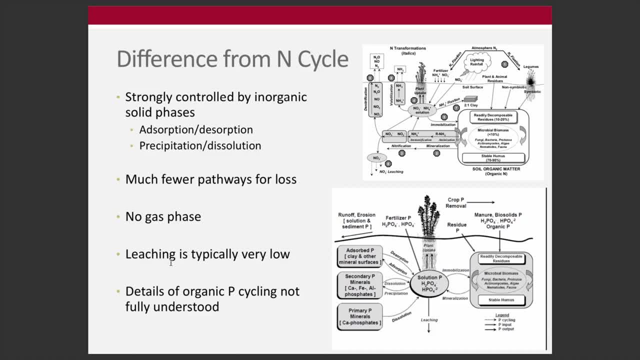 to manipulate and study For phosphorus? it's not, you know, there's no kind of stable isotope form. It's a radioactive isotope which is much more dangerous to work with and a lot more controlled and just more expensive as a result, And so part of that, you know, is one of the. 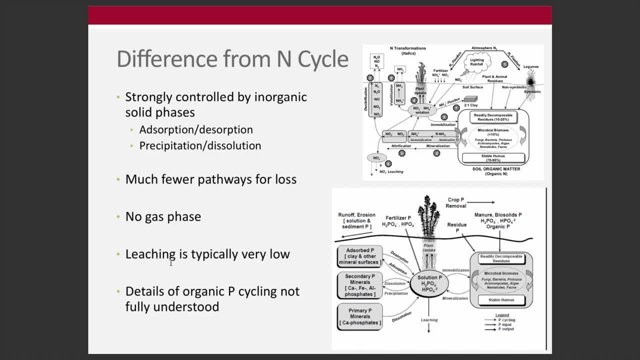 reasons that we don't have a. there's still plenty of mystery in terms of nitrogen and the controls of nitrogen cycling in the organic fraction, But for phosphorus it's even more so. Additions, transformations, losses. Really, we're going to talk. 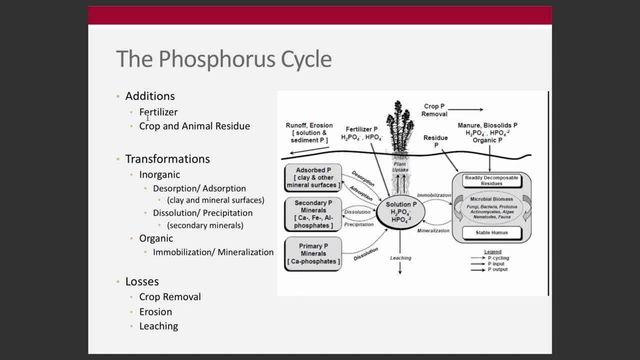 about additions. We'll talk about that in a later lecture about pea fertilizer. We don't really spend too much on erosion, leaching, crop removal- We've talked about these with nitrogen. Really, what we're going to focus on primarily is this transformation piece. 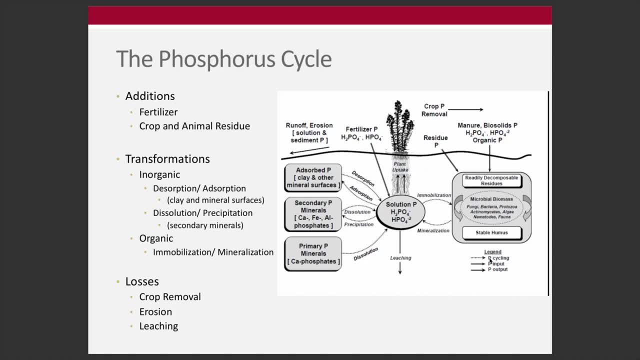 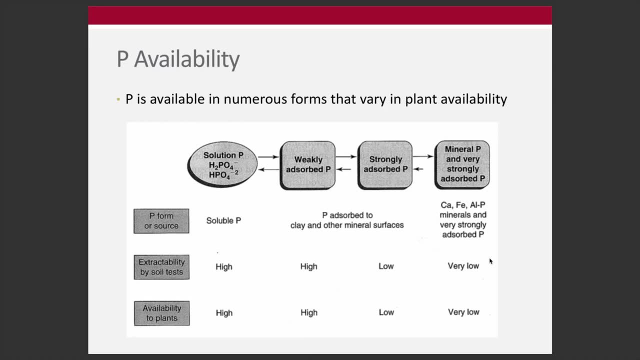 and looking at these kind of three components here. So that's what we're going to get into now. Phosphorus is complicated. Phosphorus cycling is complicated And you know we draw. we can use these conceptual diagrams, like you're seeing here, and talk about solubility or availability. 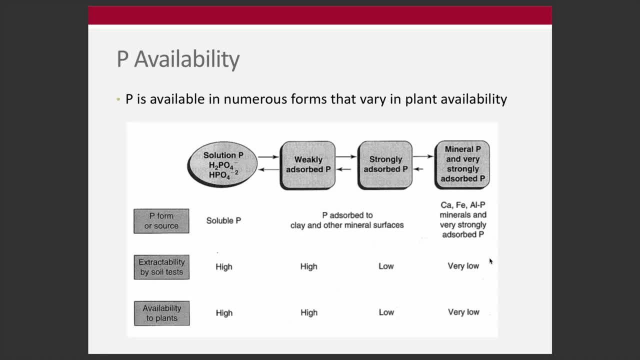 being high, medium, low, very low, et cetera, et cetera, And we typically will, you know, define these by our methods. They're what we call operationally defined, which means that our method is actually defining what that pool might be. So we might think of solution P. 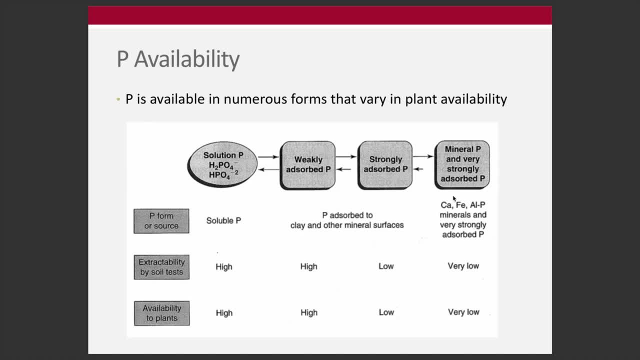 weakly absorbed, strongly absorbed and then very strongly absorbed, And we might have some of these successive fractions that would quantify that right. And that's for phosphorus. there are several fractions that do that. A headly fraction is one such thing, But you know. 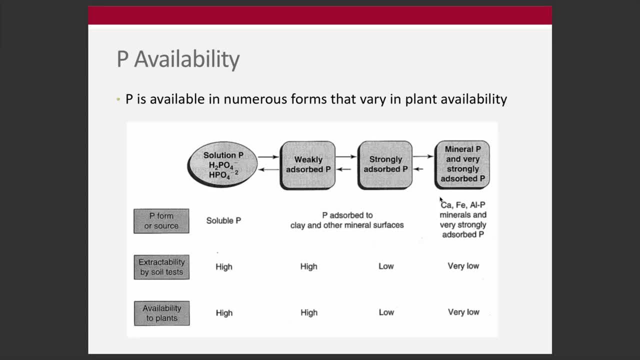 we can again classify these things into these nice clean boxes. The reality is that there's a lot of overlap and we just, you know, have to often say like, okay, so weakly absorbed phosphorus is defined by this extraction method, for example. So that's typically what happens And we can think: 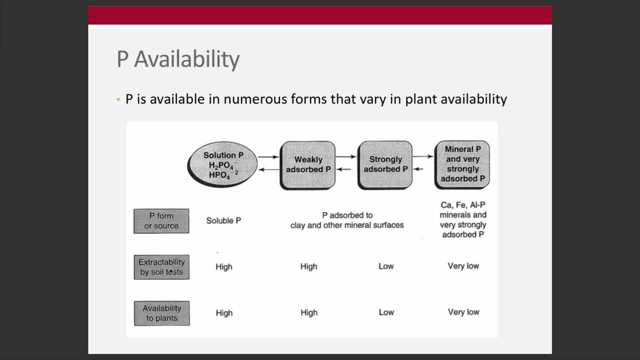 about the form of the source of P, the extractability by soil test and the availability of plants, And so really we've got solution P and then we've got this weakly absorbed P. Both we would consider those highly available, And then we've got this kind of strongly adsorbed 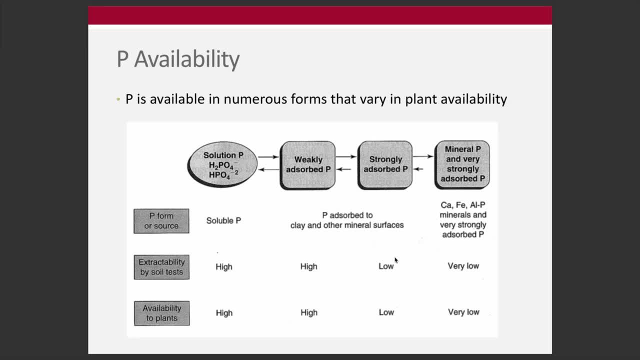 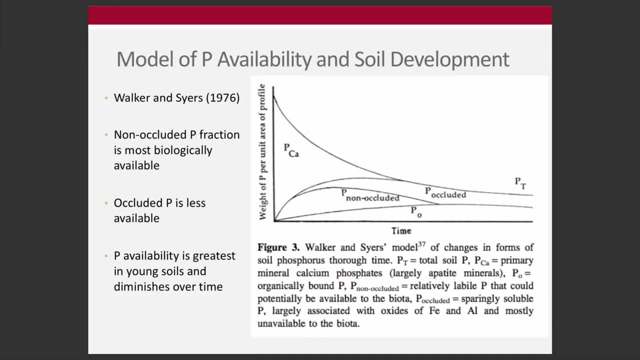 and then even into the mineral fraction, And then this is like, becomes available. okay, Now an important model, an important model for phosphorus development, soil development, is. this was proposed, you know, over 40 years ago by Walker and Syerson. 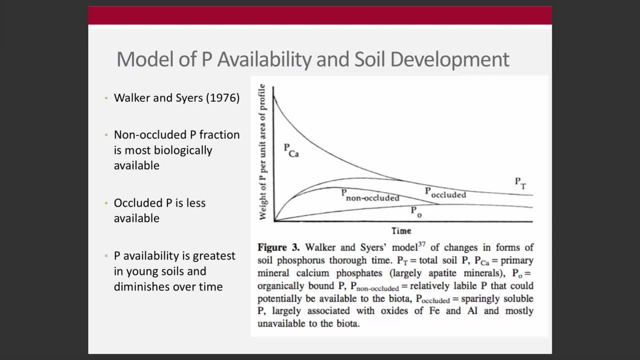 And it's this idea of kind of soil weathering and then the form and fraction of phosphorus that occurs, okay, And so this is again from their original public publication And this is really a percentage of that phosphorus fractionation. 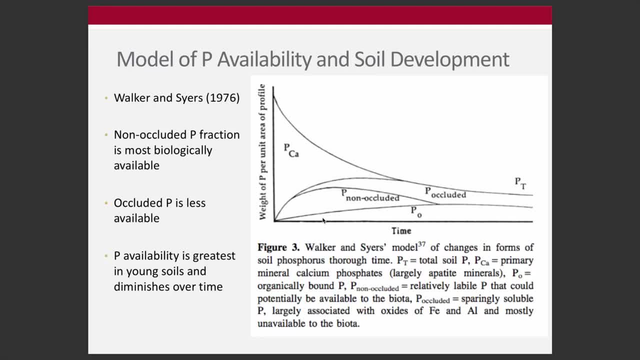 or phosphorus piece over time, And what they proposed was that soils that were young, relatively recently developed, would have this non-included phosphorus fraction. that would be highly available and occupy. you know, if you added all these up, it occupies this P subscript. 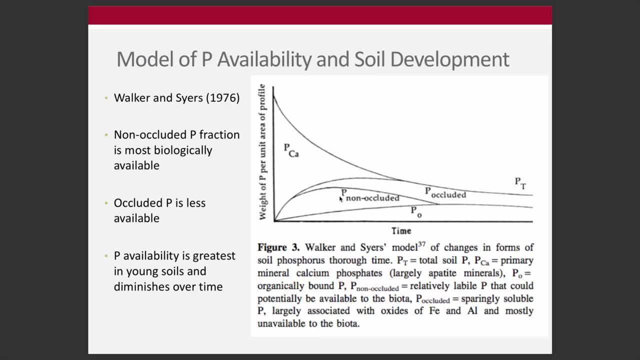 non-included- occupies a large percentage of the total phosphorus, As that soil would age. over time it becomes less and less until it basically becomes really hard to measure, And then it's taken over by this occluded phosphorus and then this organically bound phosphorus is kind of like 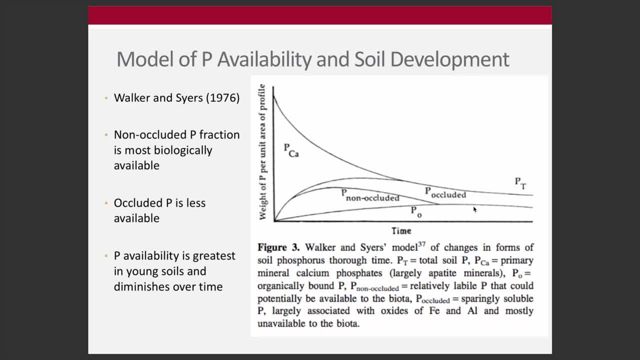 this constant piece to this whole time series. okay, So what they hypothesized was that phosphorus availability is greatest for plants when soils are young and really this diminishes over time. okay, And so you know, this is an important kind of model if you, you know, are studying phosphorus. 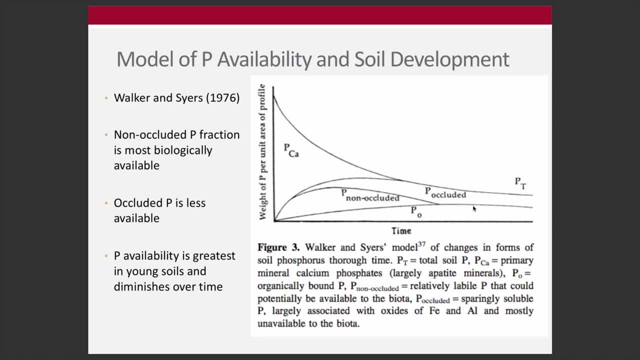 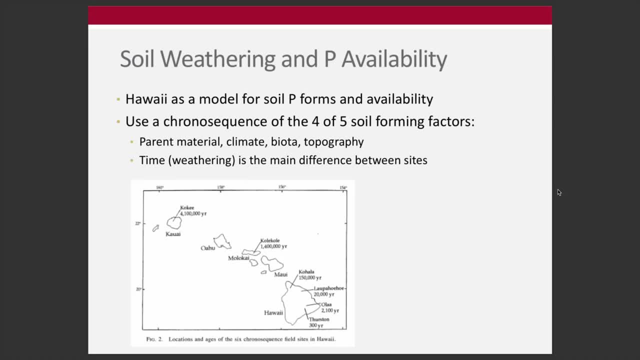 and really kind of getting into some of the science behind it. this is something to be aware of And there's been great work that's, you know, kind of taken this theory and shown it. you know some empirical evidence for it And I just point out that you know one of these examples is Hawaii. 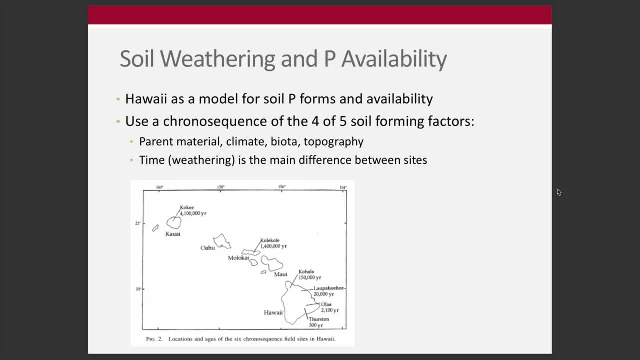 as an archipelago and a set of islands. that you know is pretty much a pretty small island, but it's. I think it's about a hundred kilometers from the bottom of the ocean and it's sort of a really nice. 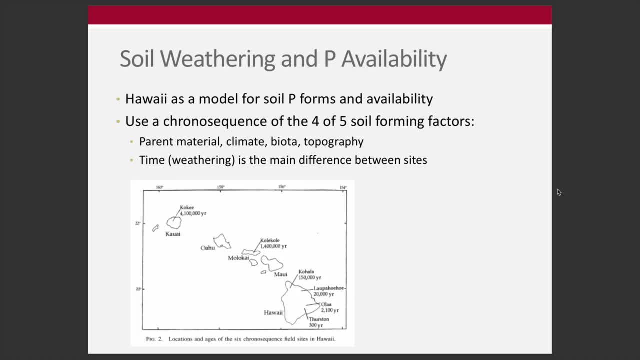 it's kind of a really nice natural experiment as a chrono sequence. okay, If we think back to, you know intro soil or the five soil-forming factors from Hans Jenny, it's parent material climate, the type of biology that's here. 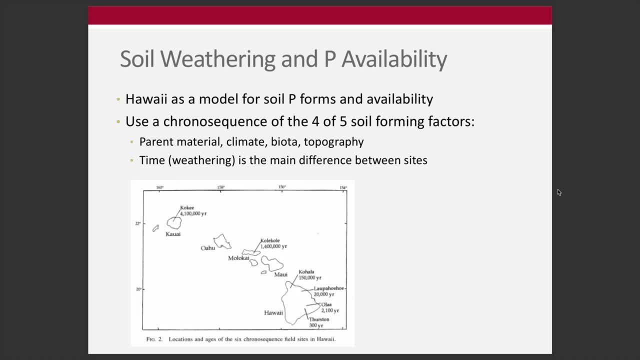 the topography, and the last one is time: how much weathering has occurred, These five things right, and animals and soil critters that are there, how steep the slope is, and then, this time or weathering piece, these things, these five pieces to a large extent determine, uh, what type of soil. 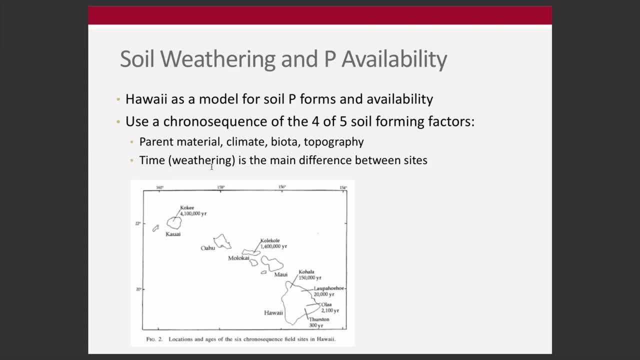 we have and that's. you know, that's just kind of a soils 101. you're going to get that and you know, if you haven't taken a soil intro soils class, that's one of the first things you talk about in terms of um what, what creates um soils and what determines what type of soil we have. okay, 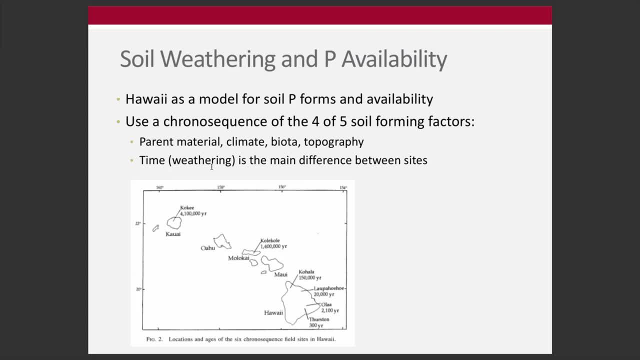 so hawaii is a really nice example because a lot of these things are controlled, for we have islands that are over four million years old, a million and a half years old, say 150 000 years old, and then even new pieces of that island, as this, you know, plate has. 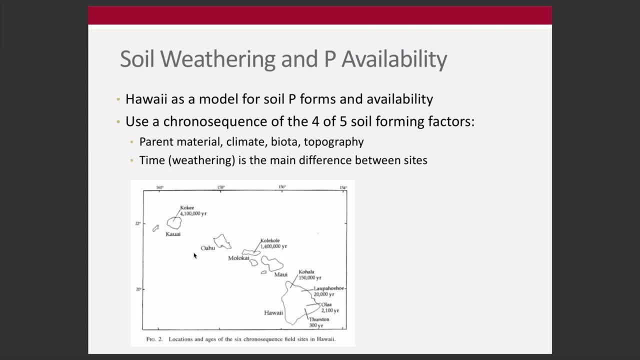 shifted in. this kind of volcanic activity has has bubbled up from the surface and formed these islands. we've got soil in hawaii that's less than 300 years old, so this is like the most recent piece of that island versus the oldest and in terms of where that, what is in that parent? 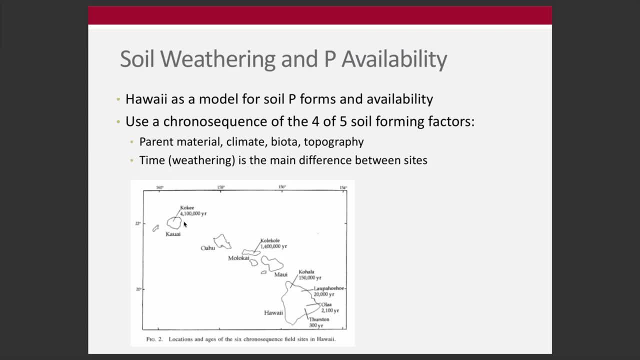 material, the climate, the bagger, the biology and the topography. we can really control those. hold and look at time as our factor that we're manipulating. okay, so that's a nice model. this has been used, uh, for a lot of ecosystem ecology and a lot of biogeochemistry studies. 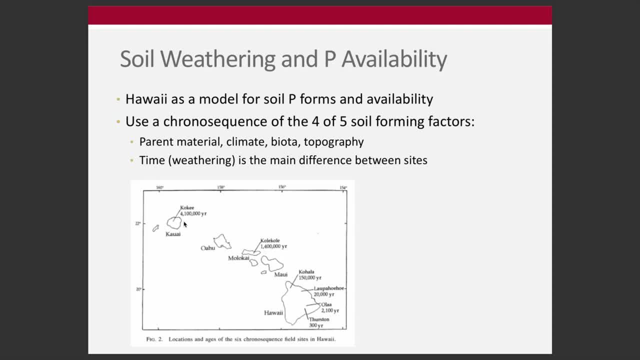 um, peter vatusik at stanford has, uh, you know, made his whole career really kind of studying this as a as a model, and there's been lots, of, lots of his students and scientists that have come and looked at different components. so it's, it's a pretty interesting thing to 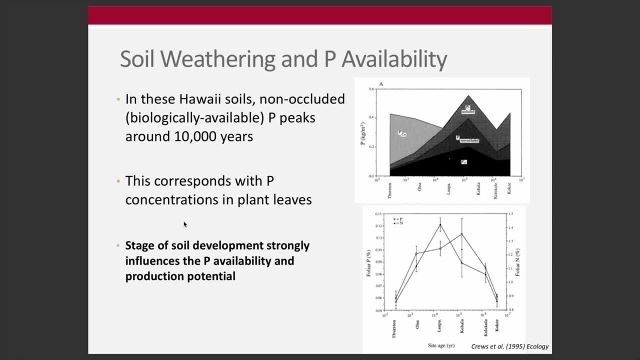 start to dive into. so, soil weathering and p availability. um, in hawaii, soil is not included biologically or not included. that is biologically available peaks the amount of of that non-included phosphorus fraction peaks around 10 000 years. okay, so, uh, this is you know from a 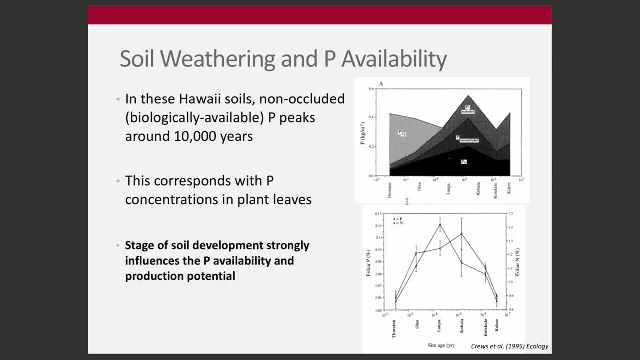 study done several decades ago, but very, you know, very important, highly cited studies showing the time from very young to very old and then looking at quantifying the different phosphorus fractions, from calcium-based to organically bound, to occluded and non-occluded. 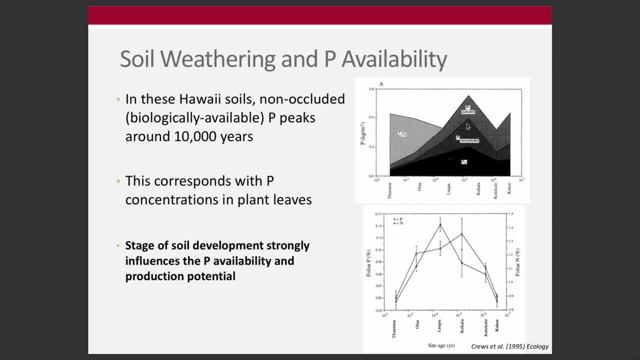 And again we see around 10,000 years is where this non-occluded piece really peaks. And, interestingly, if you go and you sample foliar phosphorus concentrations with what these authors did, we can see the phosphorus is these open circles. 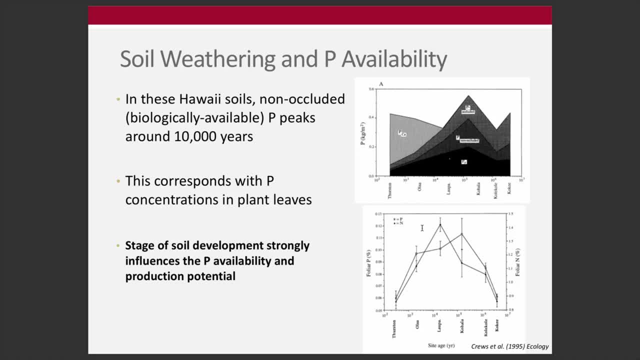 or sorry, these open squares, nitrogen being these kind of closed diamonds, if you can see that, And it's really around this 10,000 years where we see foliar phosphorus concentration increase. Now these are, of course, tropical forests in Hawaii. 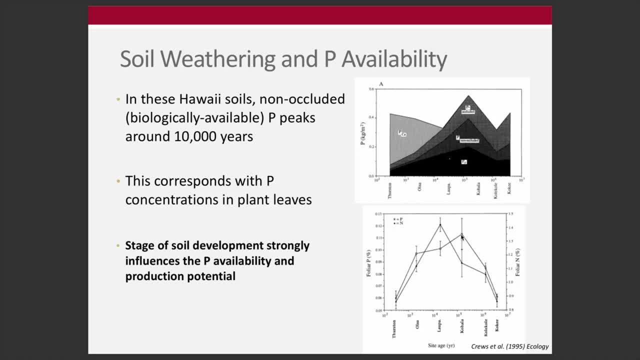 These aren't phosphorus-fertilized. okay, But it's just we're looking kind of, if we remove this element of management and remove the element of fertilizer, how much phosphorus is available and you know how is that reflected in plants and plant development? 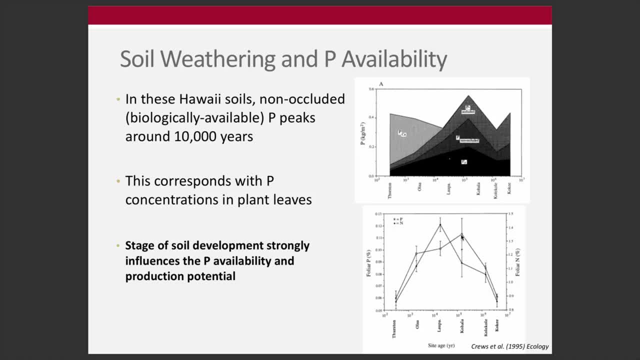 And so you know this again is kind of seminal work, showing that as soils age, phosphorus and the phosphorus availability kind of evolves, It peaks say around: well, at least in Hawaii at 10,000 years. 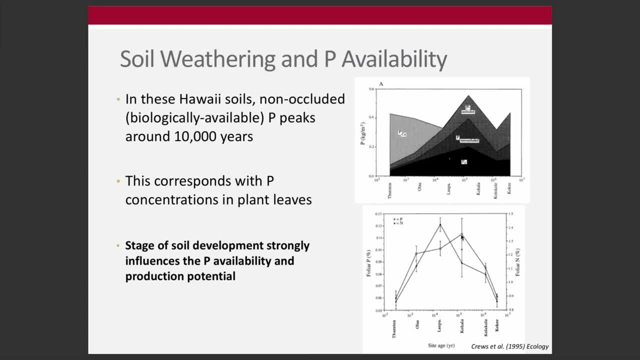 but sometime in relatively geologic time it peaks And then it starts to that availability starts to decrease over time And if we think about you know the soils that say we have here in Ohio and you know might want to compare that. 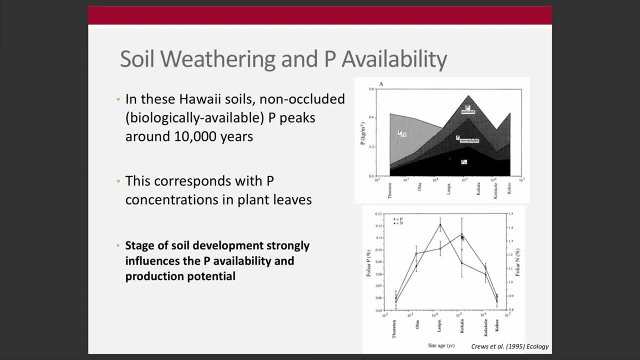 to say what we find in, say, Georgia or Mississippi, or, you know, Alabama, southeast. we have much more recently glaciated soils here, Soils that might be 10,000 years old or 12,000 years old, or you know 8,000 or what have you. 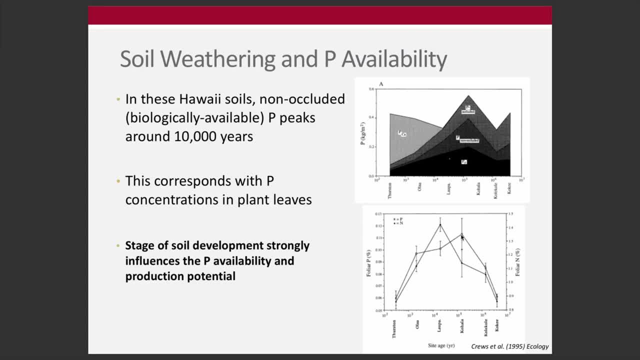 versus. you know some in the southeast where they have not seen glaciation, you know, say in the last 100 or more 200,000 years, And so those soils in the southeast are very different. Phosphorus availability is very different as a result. okay, 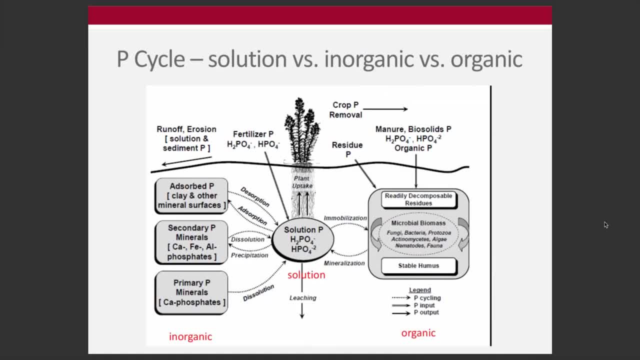 Okay, so just kind of keep that in mind in terms of you know, it's all this stuff that we're going to be talking about now. A lot of it is dictated by the age of that soil, And the age of a soil has a lot to do with how it behaves. 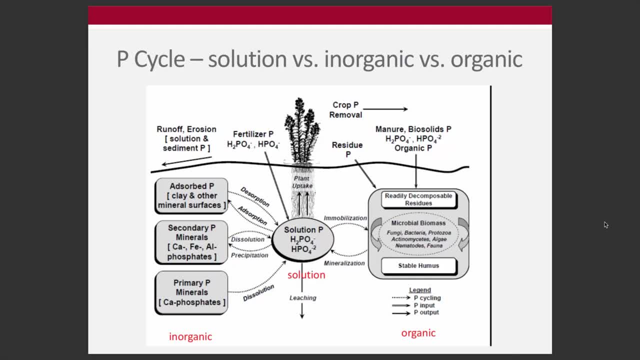 how it functions, et cetera. We talked about that early in the semester, with isomorphic substitution and negative charges and one-to-one versus two-to-one clays, And the same is true for you know thinking through some of these cycles, okay. 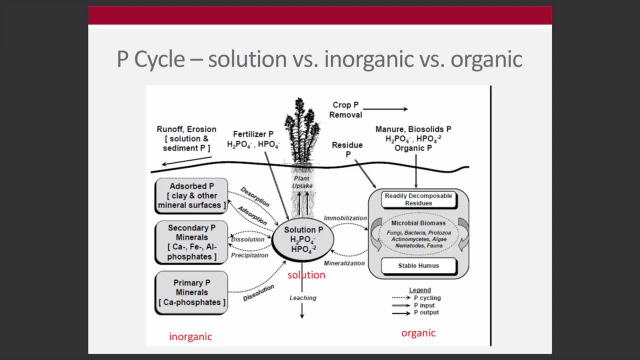 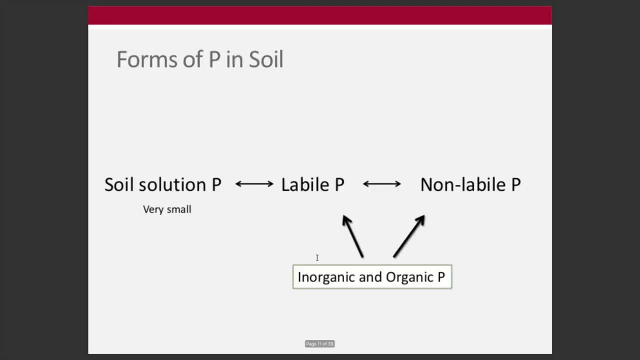 So back to our phosphorus cycle, Our inorganic fraction here, our solution and organic, And we're going to start by talking about the solution phosphorus. next Solution, phosphorus is a very small fraction, the total phosphorus, And we have labile or available P. 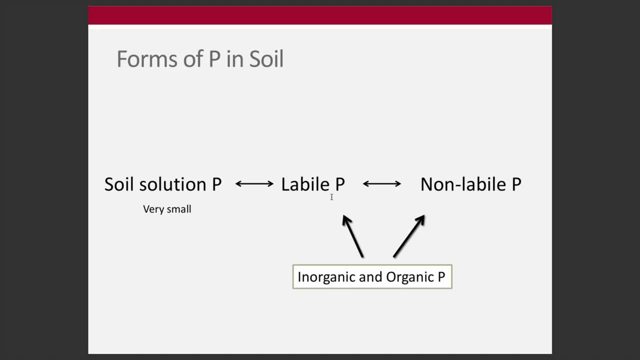 and then non-labile or non-available P. Both the labile and the non-labile are represent both inorganic and organic forms of phosphorus. So it's important when we think about availability, you know we're talking about kind of relative availability. 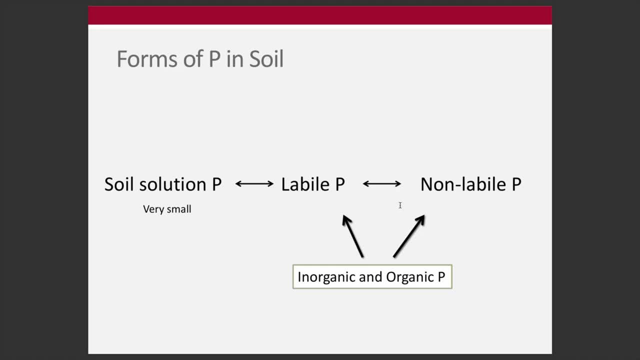 And then we're going to be talking about your inorganic first and then the organic forms of P. There'sin both of those fractions. there's relativethe availability of that phosphorus to a plant is relative, from very available to not available at all. okay, 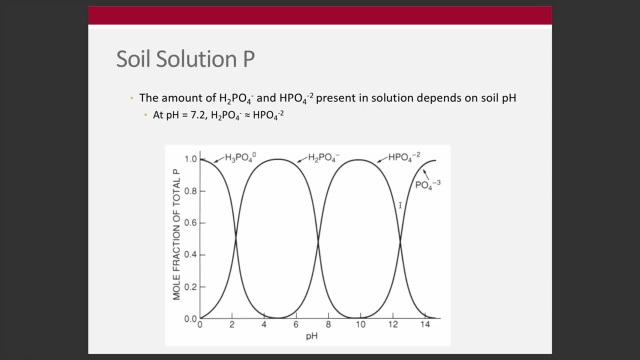 So we talked about in solution P this orthophosphate. The amount of H2PO4 and HPO4 represented in the soil solution depends on the pH, And when soils are approximately neutral, around 7.2,, the H2PO4 and HPO4 are going to be represented. 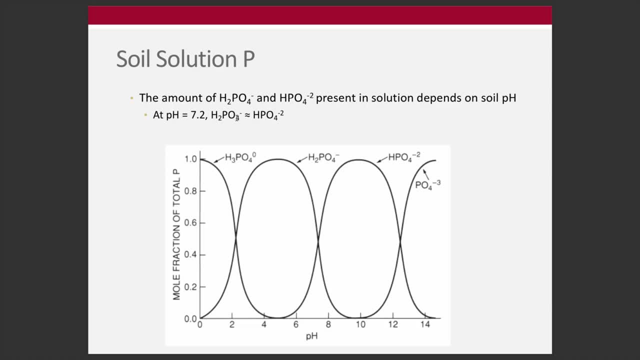 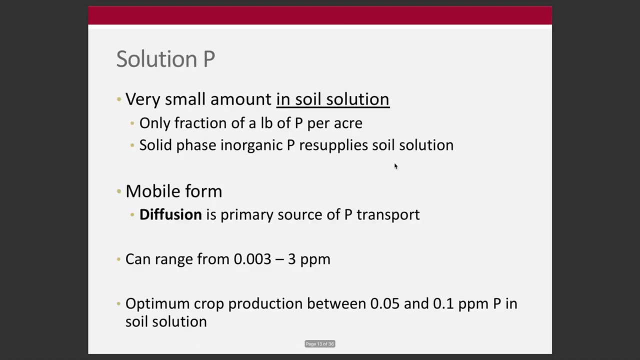 in relatively equal proportions As that pH drops. you know we can, we can see this general trend of hydrogen ions increasing, And as that pH increases, the hydrogen ions decrease, And so that's a general trend. okay, Solution P: a very small amount of phosphorus. 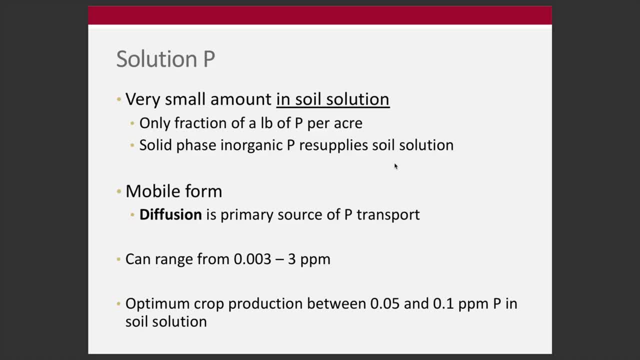 is actually in solution And when crops are plucking that orthophosphate out of the solution. you know we're looking for from a crop production perspective. we're looking for soils that are able to have a high buffering capacity and resupply that soil- phosphorus. 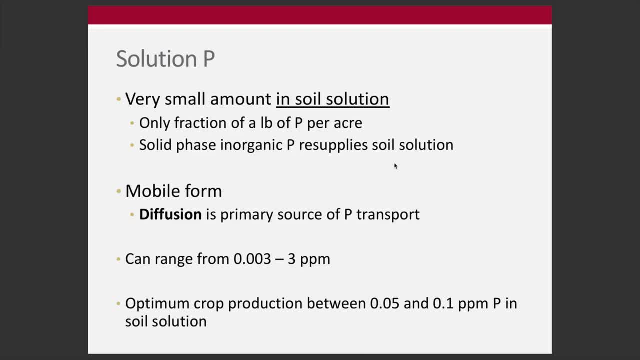 from either the inorganic or from the organic fraction. okay, Solution phosphorus moves via diffusion. We talked about this already. Diffusion is an important step and it's moving down that concentration gradient. okay, And so ranges of solution phosphorus can be .003,. 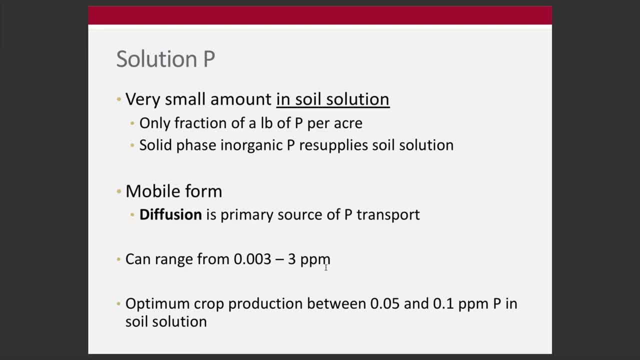 maybe up to three part per million. You can see that you know that's essentially three phosphorus molecules for every you know million, say, water molecules And that's like a very, you know it's a relatively small amount. 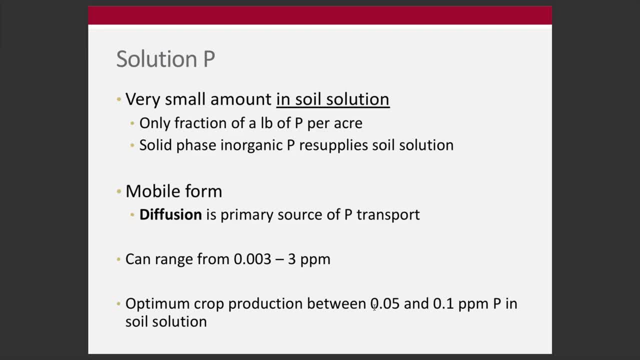 And so optimal crop production. you know this is highly dependent on the time or whatever, but a general rule is, say, from like 0.5% to 0.1 ppm is what we'd ideally like for crop production. okay, 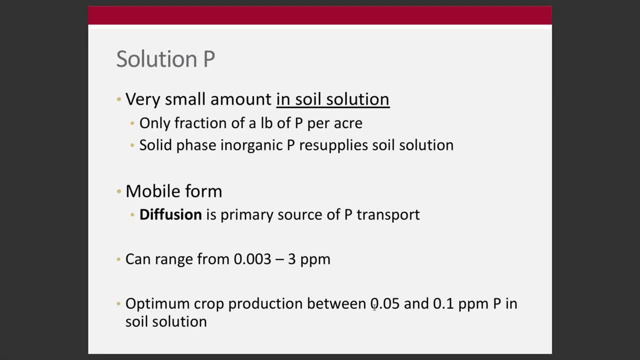 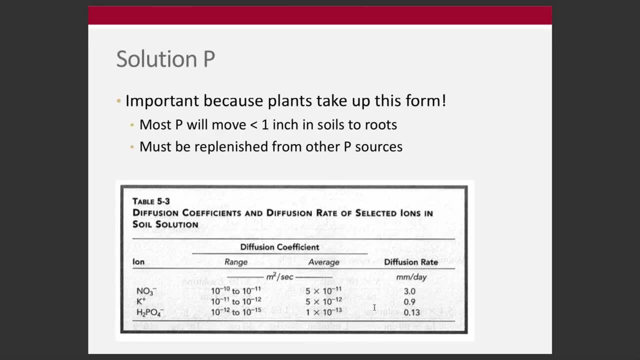 So it can range quite a bit, but it's still in a very small concentration in terms of what's in that soil solution. It's important that plants take up this form and it's important to understand that phosphorus moves very slowly in soil right. 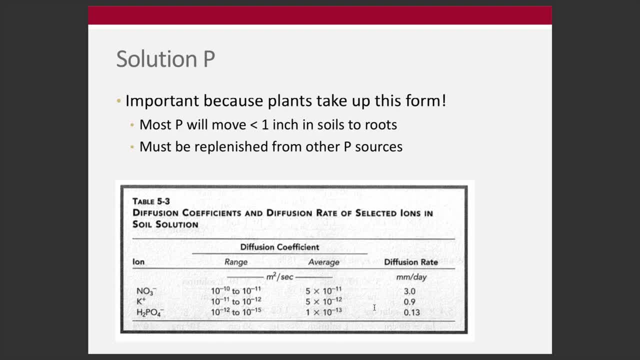 So most phosphorus will move less than one inch in the soil to roots, and they must be replenished from other sources. And so here's some diffusion coefficients of nitrate, potassium and orthophosphate, And here the diffusion rate on a millimeter per day. 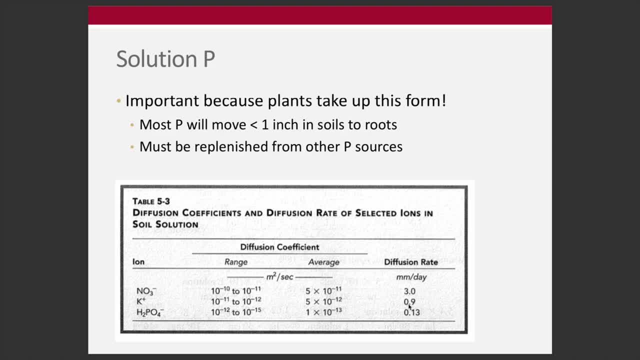 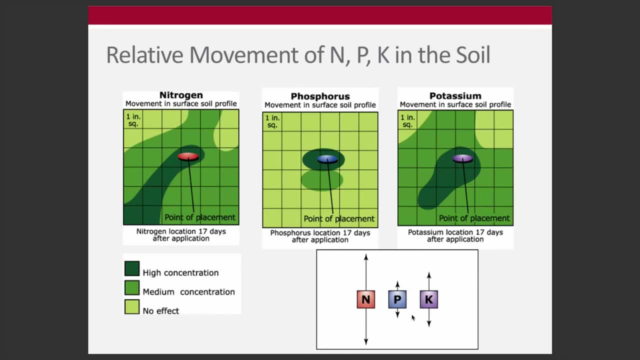 So nitrate might move three millimeters potassium 0.9, and then you can see how it drops off. with phosphorus. This is just showing the same thing from like a nutrient management perspective. where how much nitrogen if we ban, say, nitrogen? 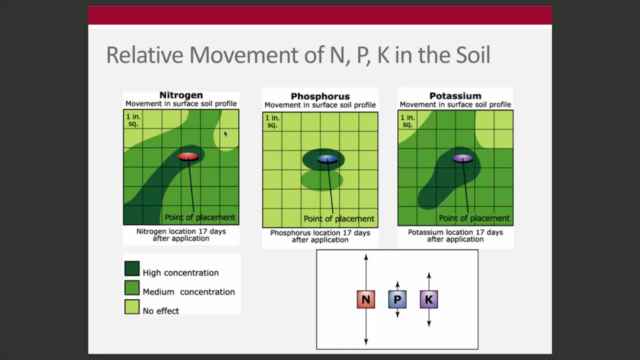 or put nitrogen fertilizer in the soil, and this is representing as up and then down right. How much movement are we gonna see? Nitrogen, we'll see a lot, Phosphorus a little And potassium a medium extent. okay, 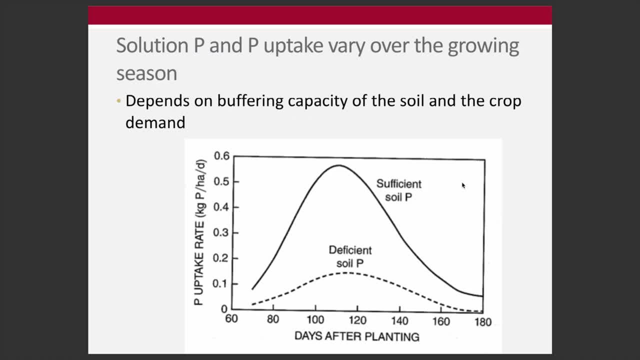 Solution P and P uptake vary over the growing season. That's, you know, not surprising. It depends on the buffering capacity of the soil and the crop demand. You know, it depends on how much is leaving versus getting removed from that solution versus how much is getting supplied. 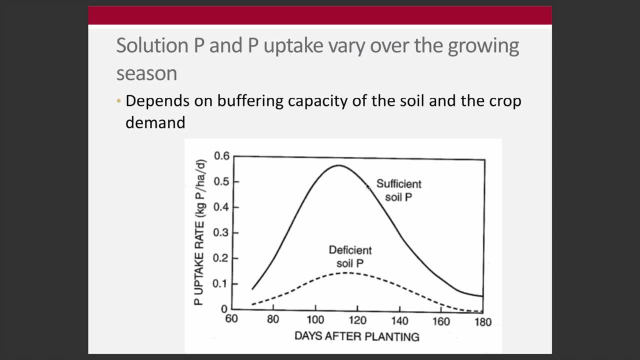 They're just showing two sufficient soils. you know the solid line being sufficient versus the deficient. This is our plant phosphorus uptake rate and days after planting And we can see that when we've got a sufficient soil, we've got a high. 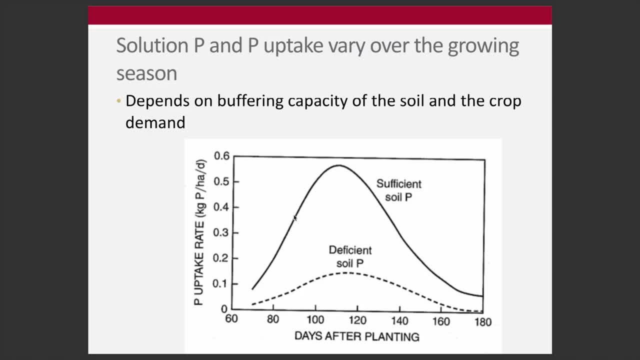 We've got a high enough buffering capacity that it can supply and keep up with that plant demand For the deficient soil. we don't, and that's you know why definition is called deficient. All right, now we're gonna talk about this inorganic fraction. 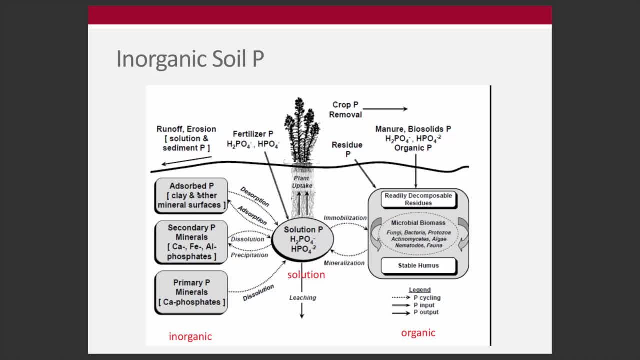 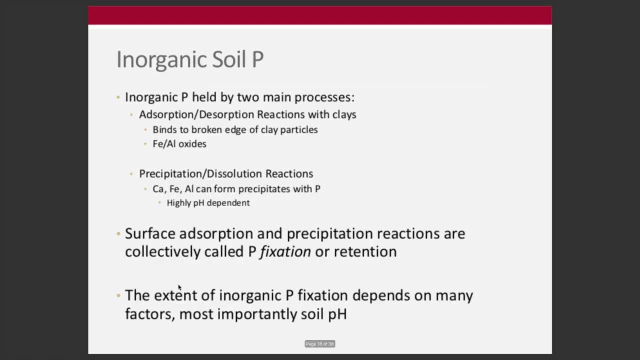 Okay, so these boxes over here adsorb P, clay and other mineral surfaces, secondary P minerals and then primary P minerals. okay So inorganic phosphorus is held by two main processes: It's adsorption and desorption reactions, and precipitation and dissolution reactions. 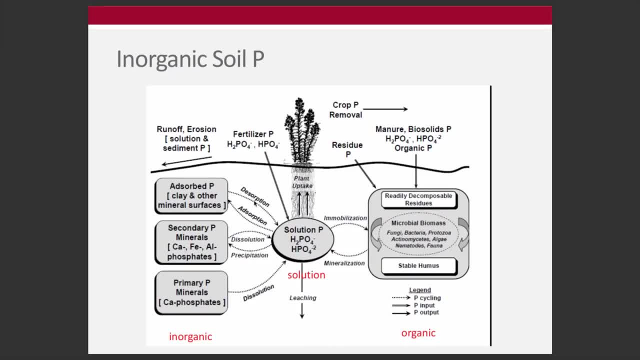 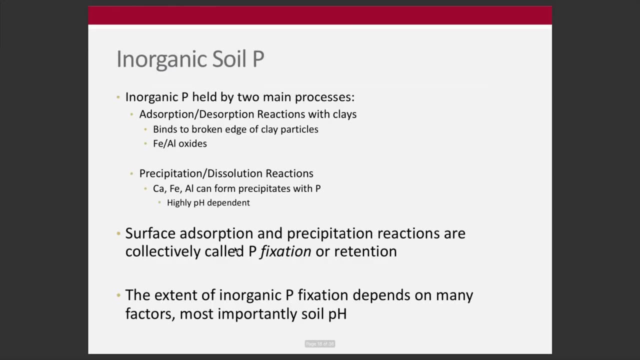 And that's what's represented by these arrows here: Desorption and adsorption. So desorption is into solution, adsorption is out of solution, dissolution into solution and precipitation out of solution. Okay, so these are the two primary mechanisms. 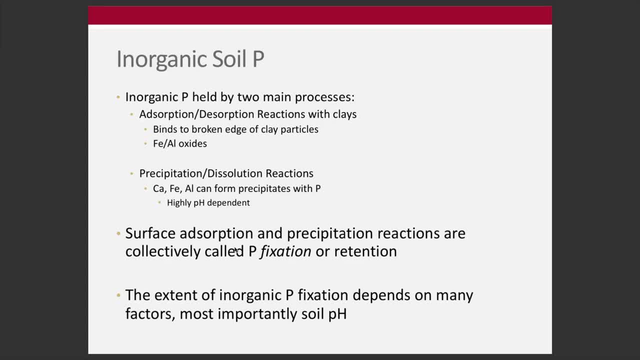 So adsorption and desorption are reactions really with clays. okay, So we think about these with clays and we can think more about this kind of in terms of exchange sites. Now, one of the things you'll notice is that 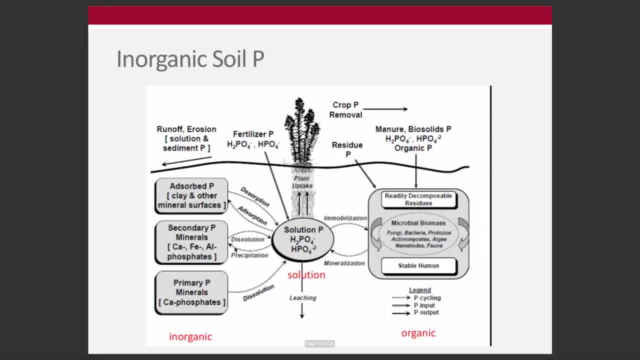 oops, pardon me, that these orthophosphates are negatively charged And we might say, oh well, you know these are negative anions and so they're not gonna be sticking to. you know these exchange sites in clays. 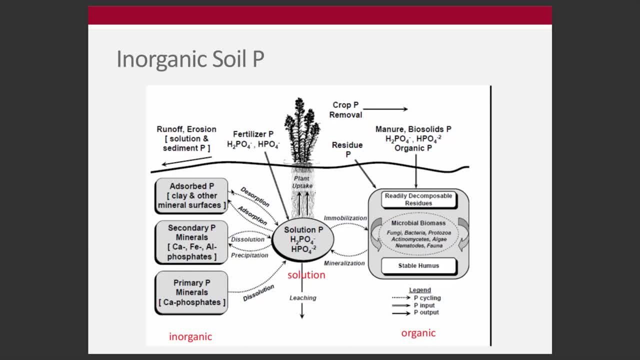 like, say, calcium or potassium would be, And that's true. but when we think about phosphorus, we're often thinking about exchange sites and you know, holding being bound to these clay. The interactions of clay and mineral surfaces are a little bit different. 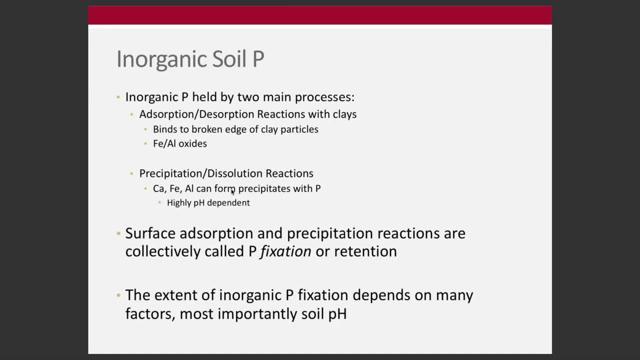 and we'll get into that in a second. okay, So rather than just the overall charge, we're typically gonna be binding to broken edges of clay particles and then iron and aluminum oxides is the primary mechanism. okay, For adsorption and desorption. 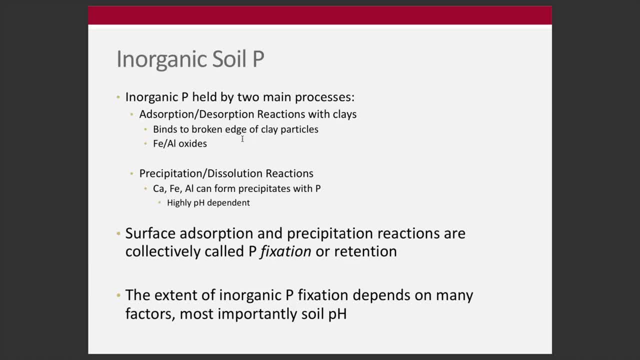 Then we've got this other piece, which is precipitation and dissolution, And these really are reactions with calcium, iron, aluminum, manganese, some of these, and they actually form precipitate, Precipitates, which are moving out of solution and into solution, depending on which way. 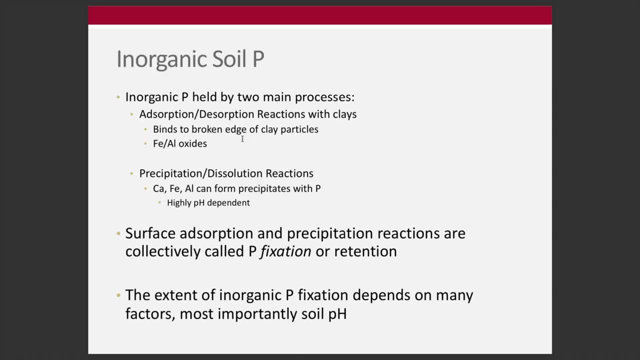 that reaction is flowing. These are highly pH-dependent, okay, And so when we talk about phosphorus, pH is a main part and we'll get a little bit more into this. okay, But pH dependency with precipitation and dissolution and adsorption and desorption reaction, okay. 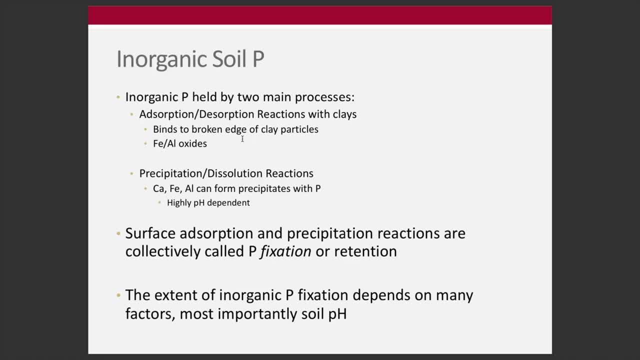 So collectively, those two processes are called P-fixation or sometimes P-retention. okay, The extent of inorganic P-fixation depends on many, many factors, but pH is a big one, especially when we talk about phosphorus. okay, 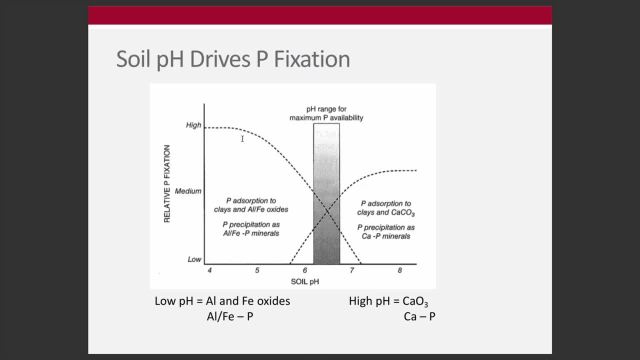 So let's get into this a little bit. pH drives soil, pH drives P-fixation and we showed in the very beginning of the class, when we're talking about acid and bases, that phosphorus is highly pH-dependent and managing soil pH is highly pH-dependent. 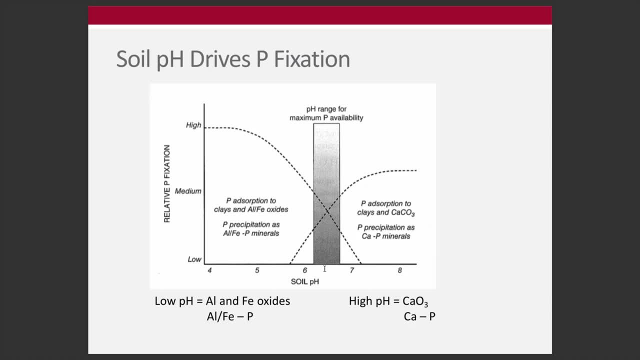 is having the highest levels of phosphorus in soil in you know an optimal pH, and it's about the best thing you can do for phosphorus availability. When pH drops and becomes acidic past six, we have a lot of reactions that are aluminum. 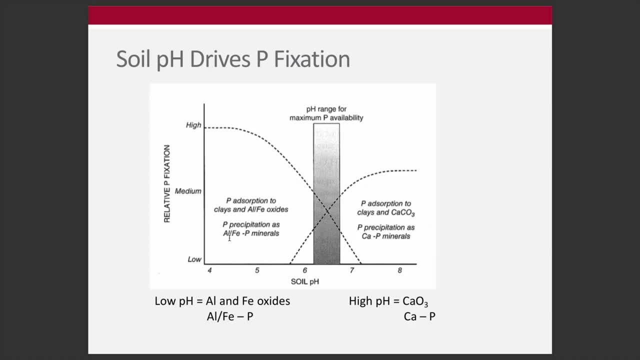 and iron oxides. There's other oxides that form two, manganese oxides being one of them, But typically, in terms of the majority, it's aluminum and iron oxides. And then, when pH of a soil turns alkaline, we have a lot of calcium carbonate that forms okay. 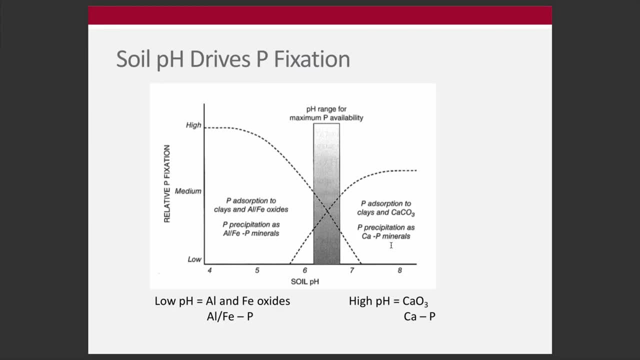 So then we have these calcium phosphates that form, And so again adsorption, precipitation, reactions on both sides, But depending on the pH, the mechanism or the actual reacting elements change from iron and aluminum when they're acidic to calcium primarily when it's basic. 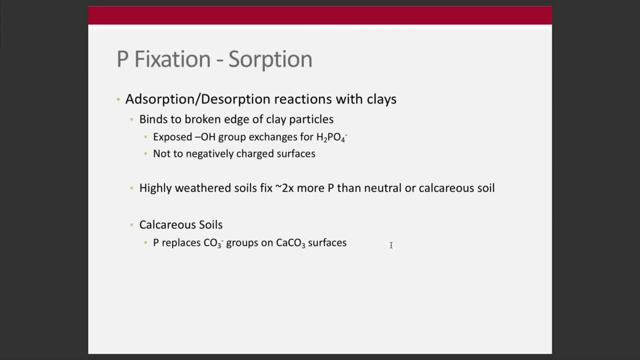 So adsorption, desorption reactions occur with clays- okay, Binds to broken edges of clay particles. So we talked about this with, say, CEC in organic matter. These exposed OH groups can often exchange with the H2PO4 reaction. 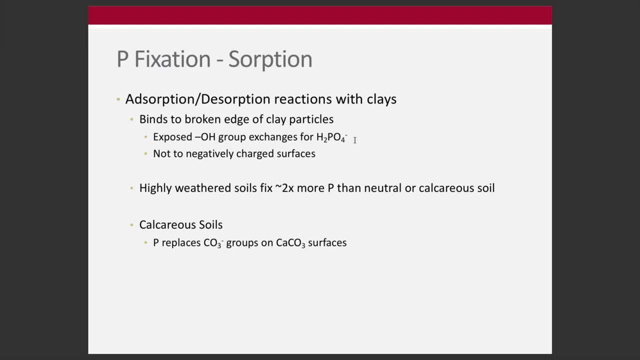 So again, the clay has negatively bound surfaces, but it's not these negative charges that are actually holding these orthophosphates. It's more like these exposed OH groups is a much larger component of that, And that's why highly weathered soils, ie 1 to 1 clays, have a lot more of these OH groups. 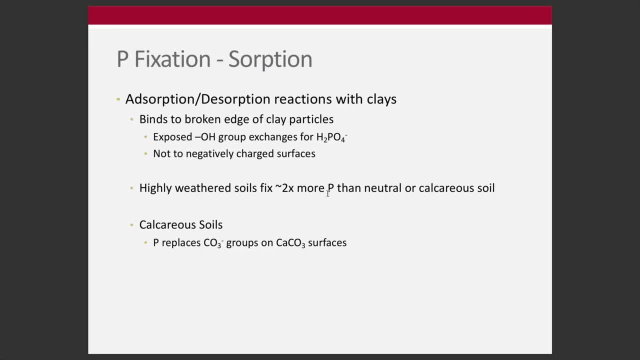 and therefore fix a lot more phosphorus than, say, a 2 to 1 clays And that's you know when we get to the point where you know we are managing, say, tropical soils or highly weathered soils. 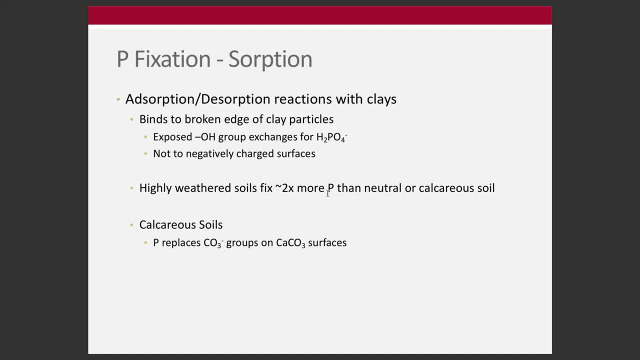 we have a lot more concern about. if we're fertilizing those soils, is that phosphorus all going to get bound up, or is it going to be available for the plant that we- you know, the crop that we plant- in the future? okay? 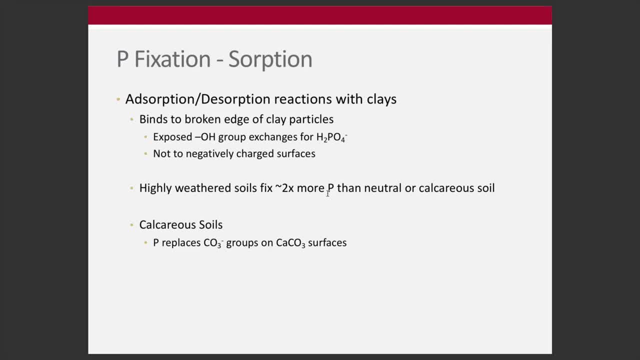 So this, you know, this idea of adsorption. desorption, it's really this interaction with these OH groups that has a large role in that, In calcareous soil, phosphorus replaces this, you know, CO3 minus groups and then forms these calcium carbonate precipitates. okay, 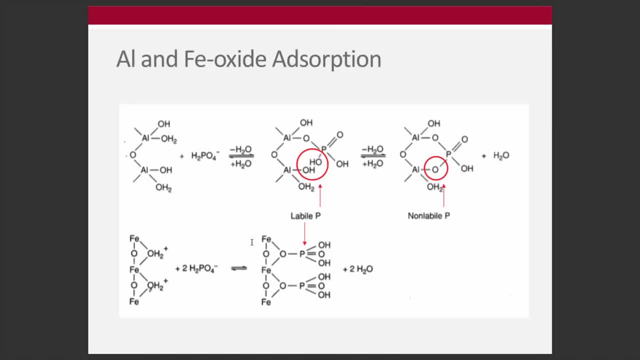 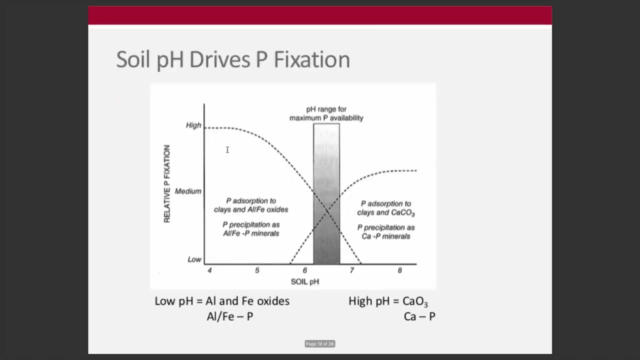 So just to flesh this out with iron and aluminum oxide adsorption, what does this actually look like from a chemical structure? Well, here we have these: an aluminum oxide, and you add phosphorus, and then you either. sorry about that, folks. 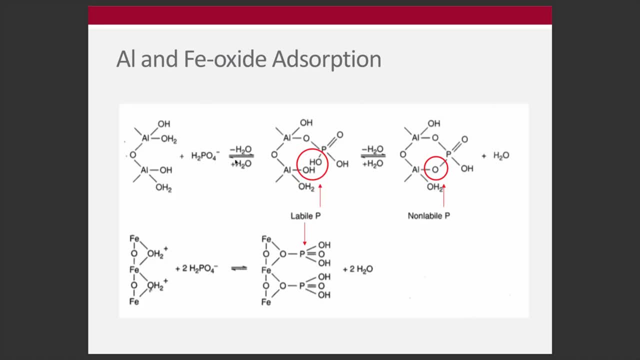 And you either. you know it's driven by hydrolysis water, depending on the reaction, But what we have here is this: you know, water that's formed, and then we've got this P2O5 that associates with these OH groups. okay, 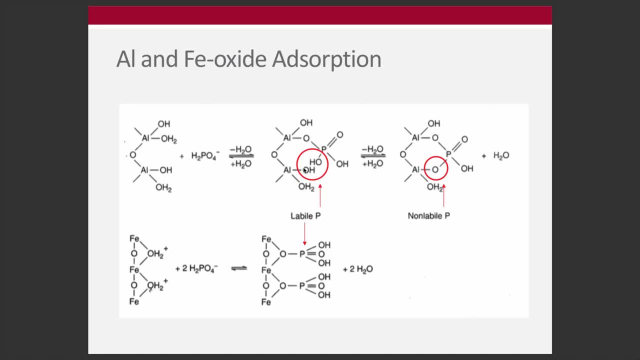 And so this is kind of bound here, but it's not like a really intricate reaction When it continues and loses Water. this one of these say, protons flows off and actually makes water and then we get this aluminum kind of. it goes from this OH, OH association. 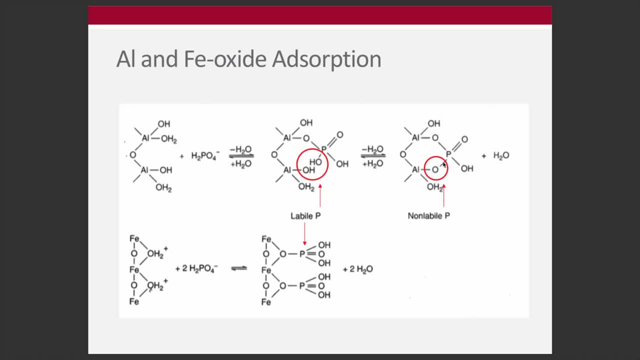 to this bound aluminum oxygen phosphorus. This becomes really fixed and non-labile at this point. So this would be considered labile phosphorus, this non-labile, So the availability decreases when it goes from this reaction to here. Likewise with iron: we've got an iron OH group. 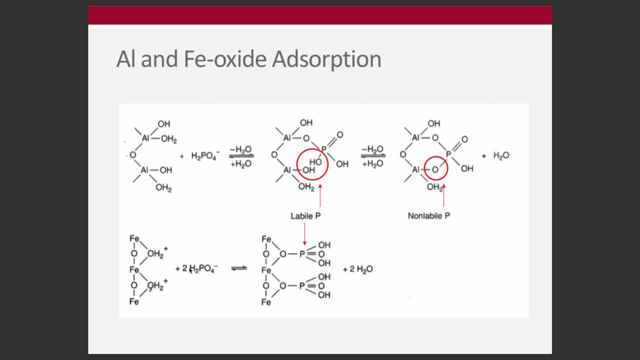 We're adding phosphorus, this orthophosphate- there's two of them in this case- And we've got that knocking that H off, that one of these protons off, and it becomes water. And then we've got this P2O that reacts. 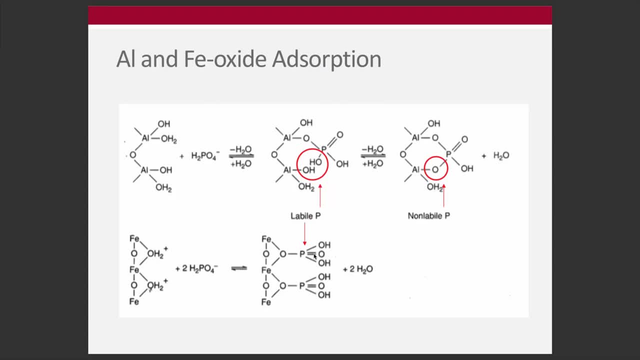 And so this would again this iron oxide would be considered A relatively labile. So this is just like. this is certainly not comprehensive. It's just an example of how phosphorus will react with these surfaces, these aluminum and iron surfaces, which, of course, occupy a huge amount of the total. 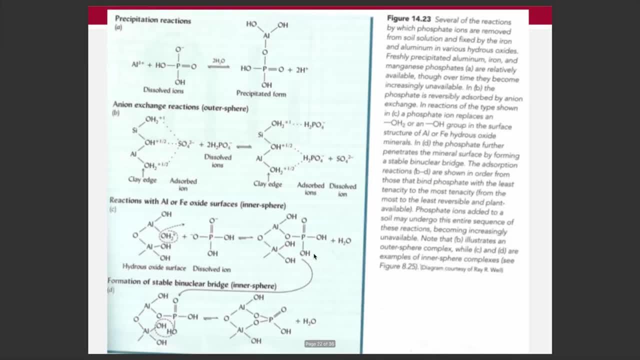 you know clay structure in soil. okay, And this is kind of an ugly diagram from the Brady and Weill textbook And it shows you know kind of the same thing. but maybe it flushes this out a little bit more. 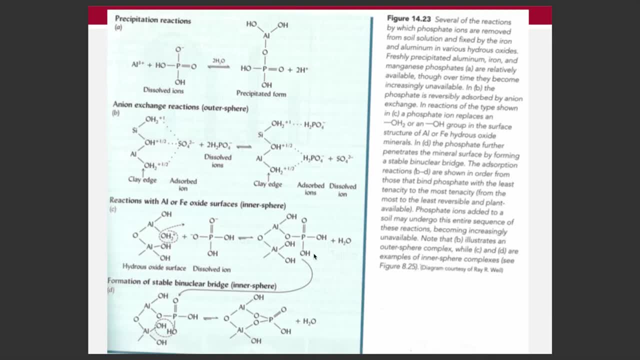 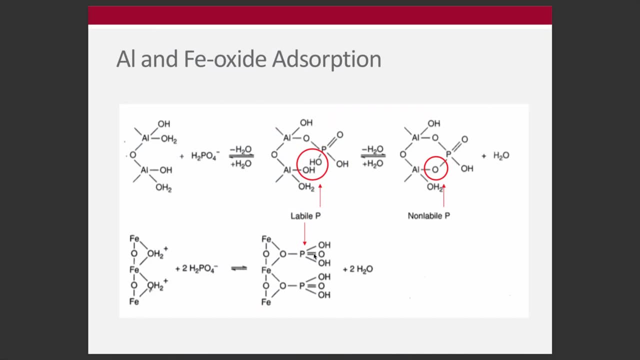 So if you're interested in looking at that to understand this a little bit better, you can. But you know, for the purposes of this class it's just sufficient to kind of understand this in a very general way. what's happening, right? 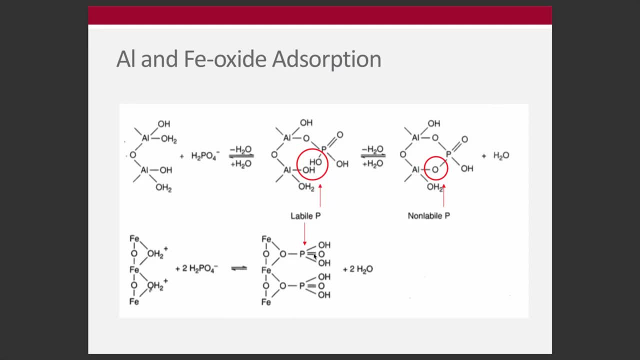 We don't need to understand the reactions, but we need to understand that they often are binding, interacting with these OH groups on clay surfaces And that's what's binding them, And sometimes it really binds them. It makes them very unavailable And sometimes it just holds them there for you know, in an intermediate state. 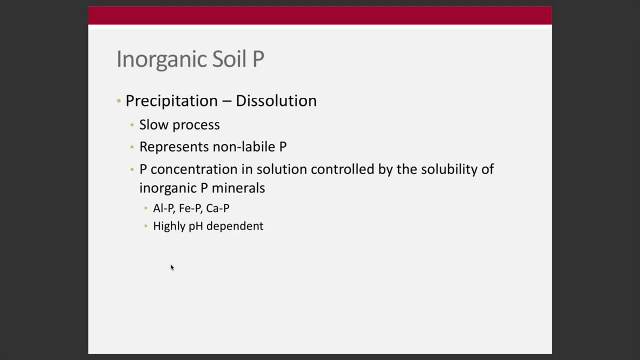 Okay. so precipitation and dissolution is another type of reaction. This is typically a more slow process And when we talk about precipitation, it's really moving that phosphorus oftentimes out of solution and making it not available. okay Again, this is the reaction that's highly pH-dependent. 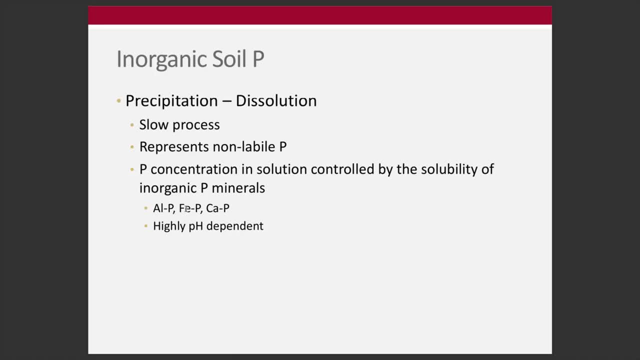 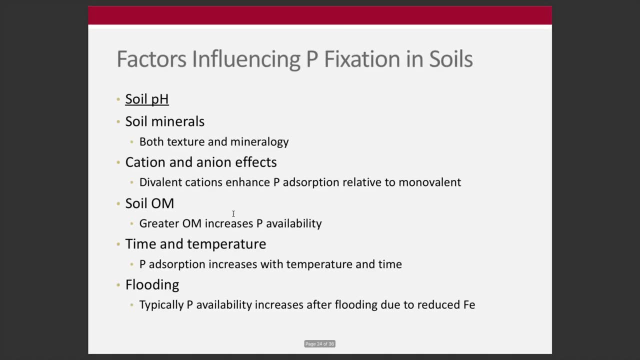 When it's acidic we'll get more aluminum and iron phosphates And when it's more basic we'll get calcium phosphates. that occur okay. So phosphorus fixation again, as the collective process of adsorption and precipitation are controlled by a number of factors in soil. 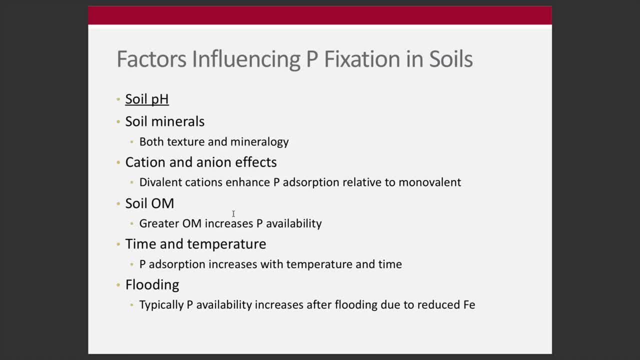 pH, pH being kind of first and foremost and one of the things that we have a lot of control over. So minerals- both the texture, like how much sand, silt and clay, and actually what the mineralogy of that clay and the silt might be- those you know have important effects. 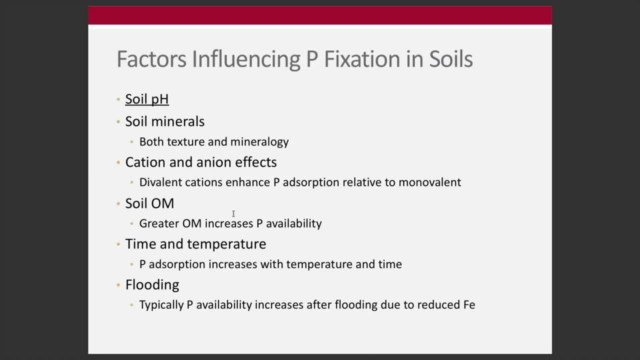 Cation anion effects. divalent cations enhance phosphorus adsorption relative to monovalent canines. So two pluses versus one plus Soil organic matter. greater organic matter increases P availability. So when we have, you know, more organic matter, we have greater phosphorus availability in plants. 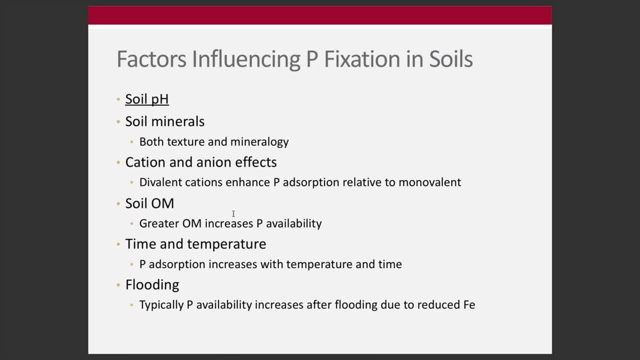 And that's, you know, should come as no surprise, right, Temperature and time. P adsorption increases with temperature and time, And then flooding events kind of cause this. when we've got these redox reactions from flooding soil and soil, 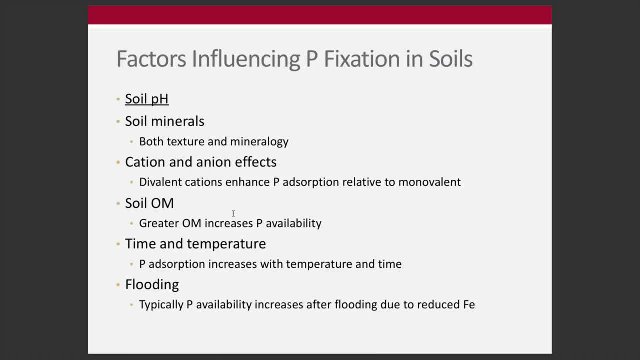 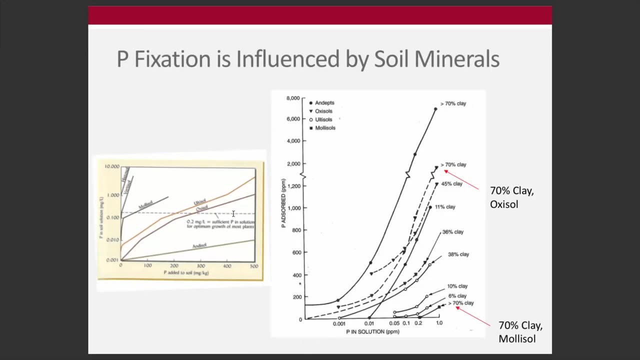 Soil organic matter. greater organic matter increases P availability. Soil has come anoxic. Phosphorus availability typically will increase kind of immediately after flooding because iron species are reduced and phosphorus, as a result, are more available. Here's just an example to show you about. you know one of these things. 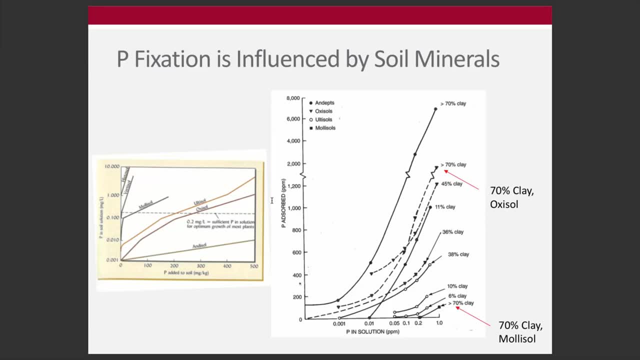 phosphorus fixation, more influenced by minerals. So here we have phosphorus added to soil. So there's soil- It was fertilized- versus phosphorus in soil solution And we can see, depending on the soil type: histosols, vertisols, mollisols. 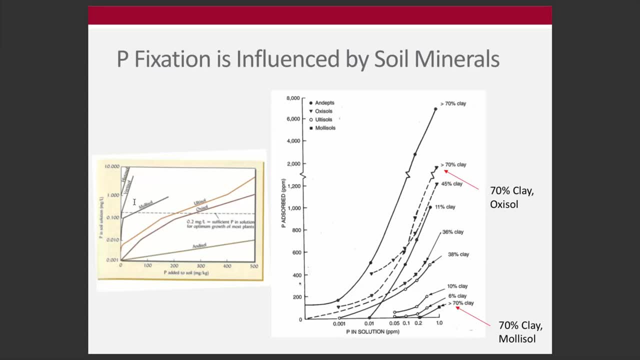 these are all would be considered kind of younger soils or higher organic matter soils, particularly these two, but mollisols also higher organic matter versus older soils. here, When we add more P, availability in these older, more weathered soils is less than in some of these. 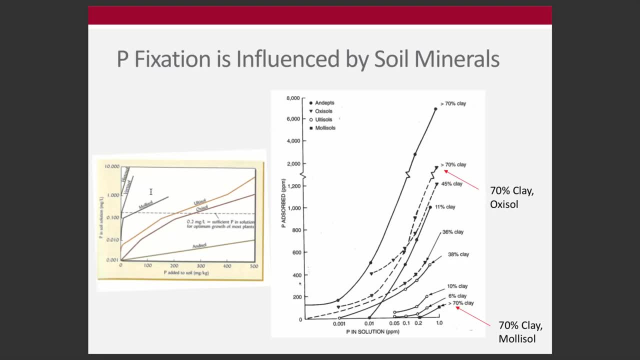 you know younger soils or soils with higher organic matter And kind of a similar thing: P in soil solution versus P adsorbed. We've got a 70% clay mollisol, so very little absorption from that, adsorption from that mollisol. 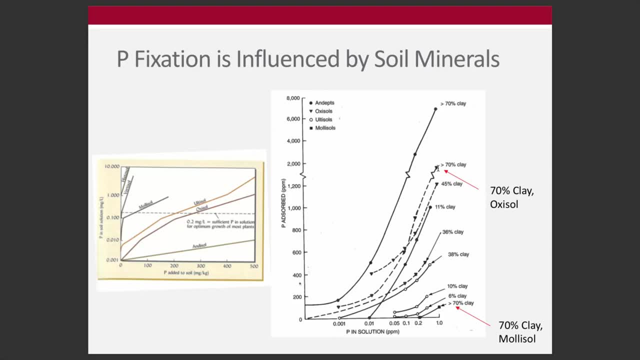 very little fixation. but when we've got a 70% clay oxosol, there's a lot more adsorption or P fixation. that occurs okay. And then here we've got an N, We've got this insecticidal which is, like you know, even higher, for example: 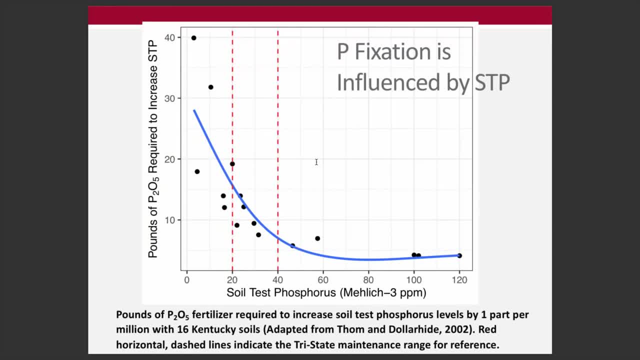 Okay To bring this a little bit closer to home and to think about this in terms of adsorption. there's a nice fact sheet from the University of Kentucky that I won't get into too much, but this is soil test phosphorus, which is a measurement of plant availability of phosphorus. 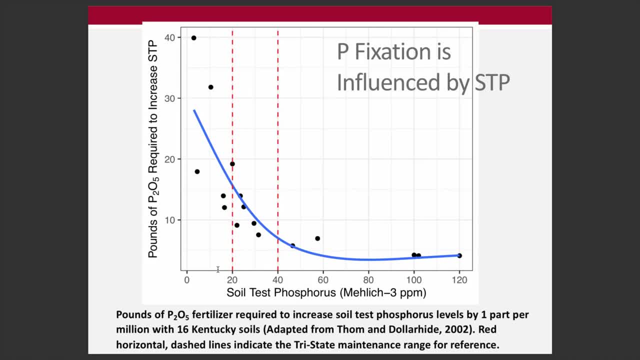 or the how available soil phosphorus is, And this is what phosphorus might be, and this is pounds of P2 of fertilizer. required pounds of phosphorus fertilizer to increase soil test phosphorus just by one part per million. okay, So what we see? the whole point of this graph, is to show that you know. it's data that's close to home. 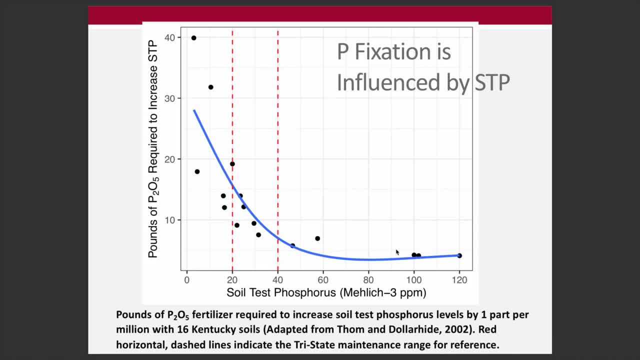 that shows that as our phosphorus availability increases, how much phosphorus is required to raise these levels even further is very small, right. So here it's less than five pounds to raise it- one part per million. But when our soil test, phosphorus levels really drop down and get really, really low. 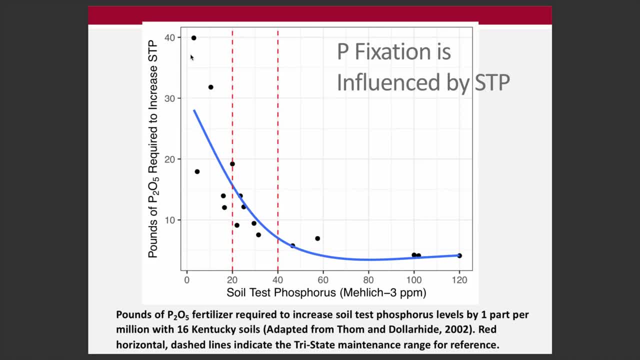 that's when it takes a crazy amount. Say you know, it takes 40 pounds of fertilizer just to increase your soil test P one part per million with this soil up here. So as soil test, phosphorus increases, as our PMS levels drop, as our phosphorus levels or phosphorus availability drops. 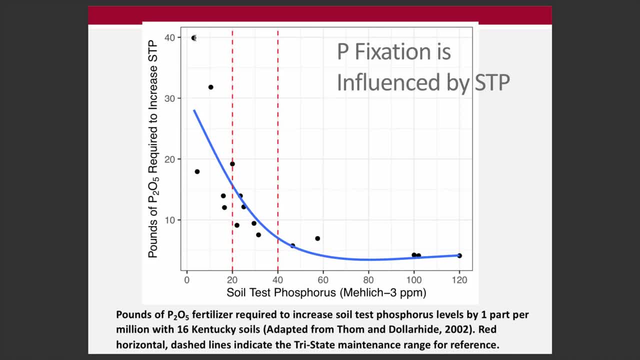 P fixation rates increase non-linearly right- And that's an important thing- from a fertilizer management and a phosphorus management. We need to understand if we're dealing with really low phosphorus soils, we might need more apply more phosphorus than we otherwise would to raise those levels. 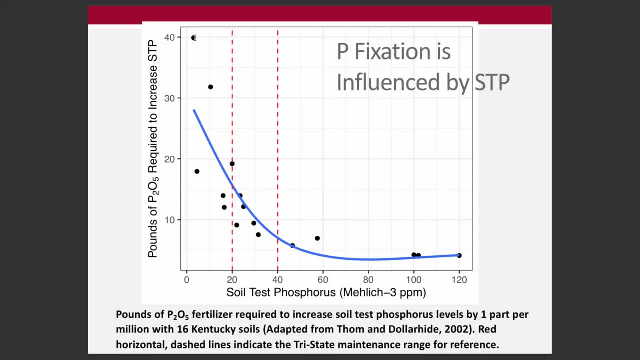 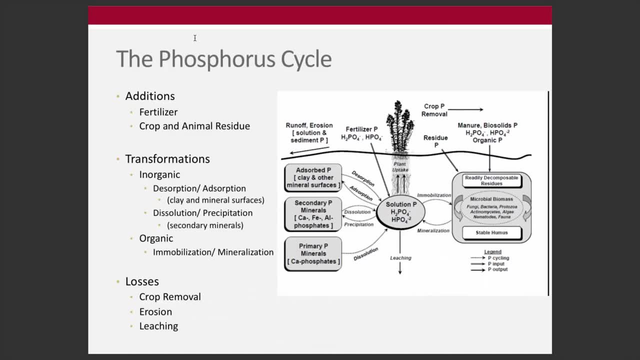 because these fixation rates are really high in low testing soils. Hopefully that's clear. Okay, so back to the phosphorus cycle. We just talked about this. transformations, this inorganic phase. Let's go into this organic phase, okay. So we're talking about not all these interactions with the mineral piece. 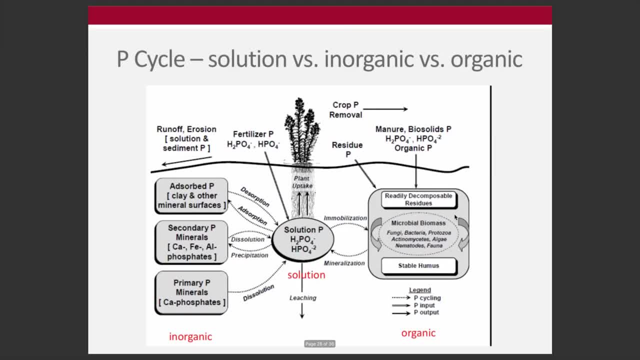 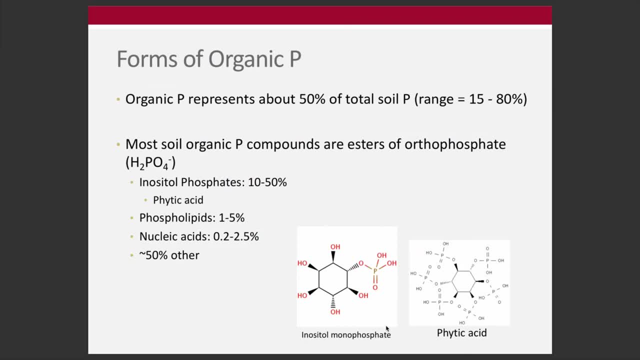 but what's going on with the organic fraction? the biology, okay, And again inorganic solution. we've covered, Now we're into the organic. So organic phosphorus represents about 50% of total soil P and that's a rough average. 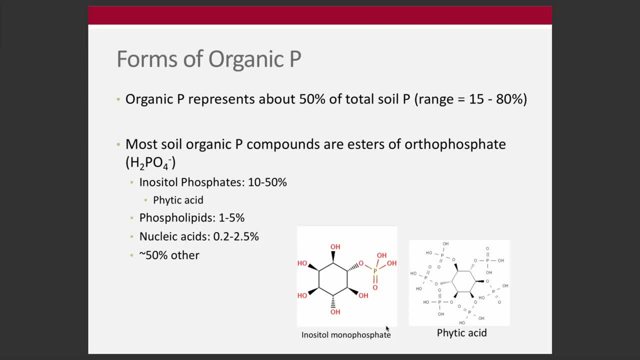